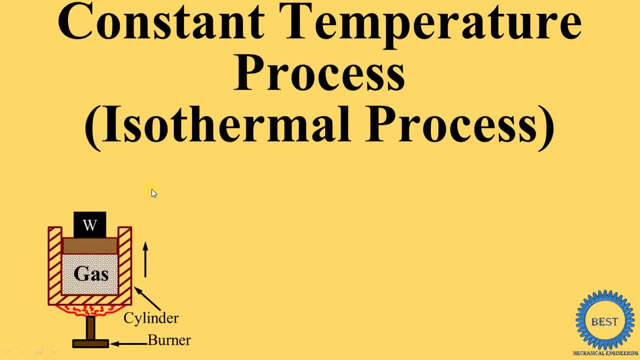 In this video I explain constant temperature process. It is also called as the isothermal process. In this video I explain basic about the constant temperature process. Then after relationship between pressure volume, temperature, heat transfer, void lamp, change in internal. 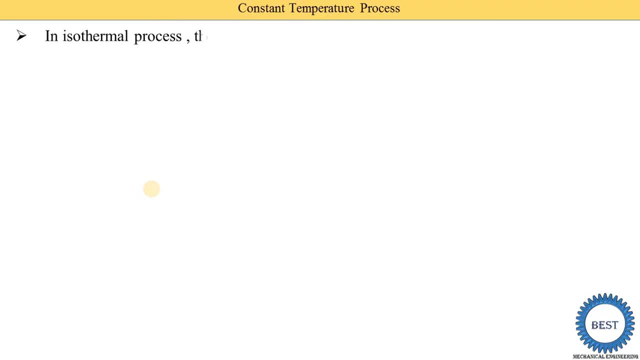 energy and the change in enthalpy. So first we understand the basic about the constant temperature process. Constant temperature process is also called as the isothermal process. So in a isothermal process the temperature remains constant during the process Means. 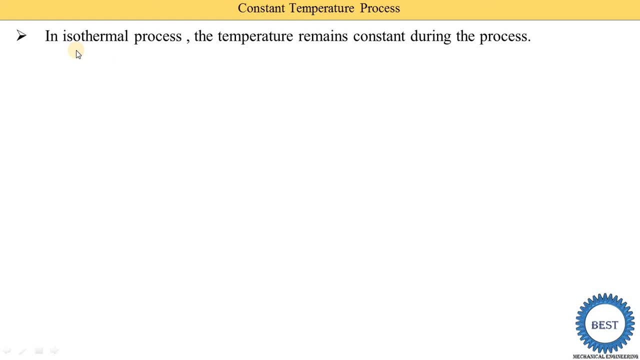 when we supply this heat energy to the gas or we remove the heat energy from the gas, its temperature is remains constant during this isothermal process. This process follow the Boyle's law. So in the Boyle's law what we consider, that is, the temperature, is remains. 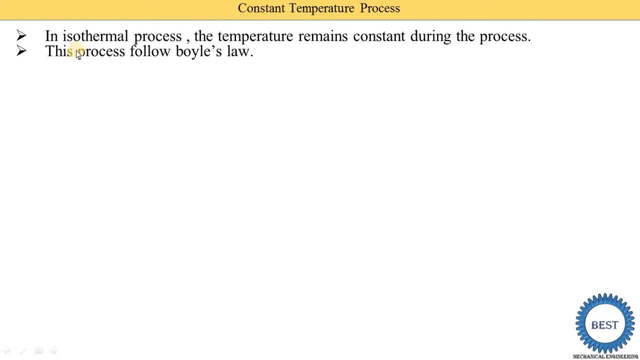 constant and pressure and volumes are inversely proportional. That means the constant temperature process is followed the Boyle's law, The law of expansion and the compression for isothermal process on the PV diagram is hyperbolic as P versus V are inversely proportional Means. P is varies inversely with the V Means. 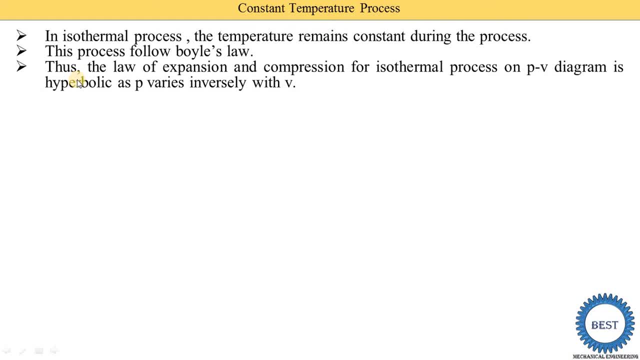 suppose the pressure is increased and volume is reduced, and the pressure is increased and the volume is increased. that is called as the inversely proportional and that the same thing we understand in the Boyle's law. So as the Boyle's law, temperature is constant and the P is inversely proportional to the 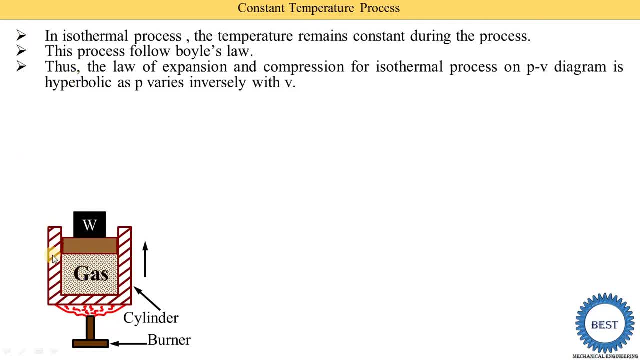 V. So here you see, this is the cylinder piston arrangement. Inside this gas is filled out and here some weight is put in, And here, by using this burner, we supply this heat energy. Ok, Now we draw this process on the PV diagram On the x axis. volume is there on the y axis. 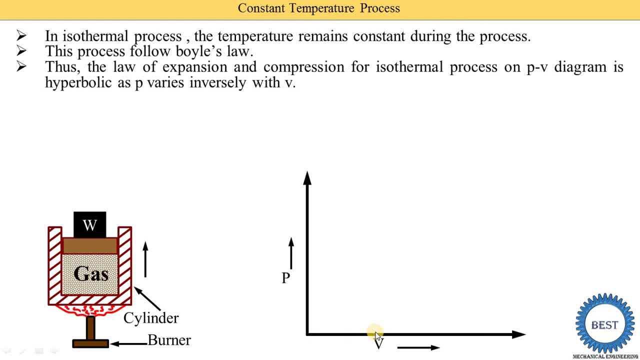 pressure is there, And this is the 0,0 points. So when we move on the right side, the volume is increased. When we moving in upper direction, the pressure is increased. So we have the volume here. When we move in the upper direction, the pressure is increased. So here we draw. 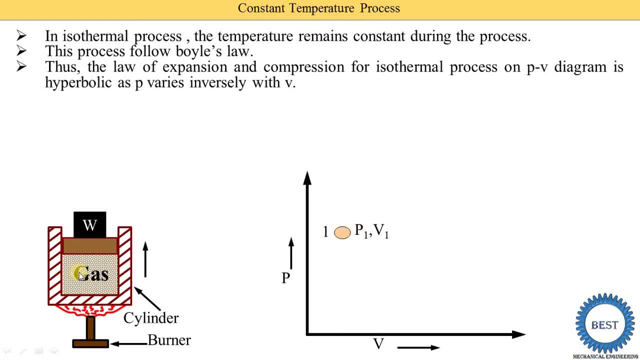 so this is the state one. okay means in this gas cylinder arrangement, that is the initial state of the gas. okay, and when we remove this heat energy from this gas means this diagram is drawn for the heat rejection process. means for the expansion process: okay, because this pressure is reduced. 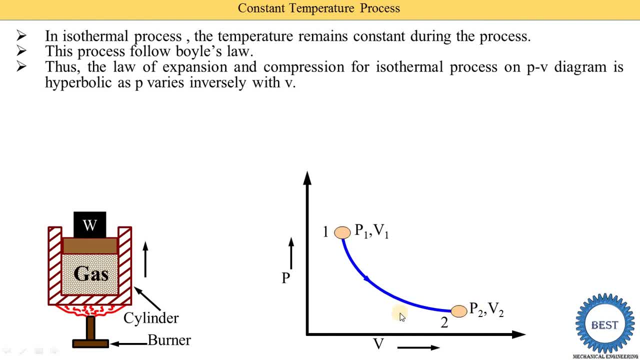 okay, so it is followed this line and we get these points here. you see, it is the pressure is reducing and the volume is increasing. okay means they are inversely proportional and constant temperature process is followed up. pv is equal to c means pressure into volume is equal to c because the 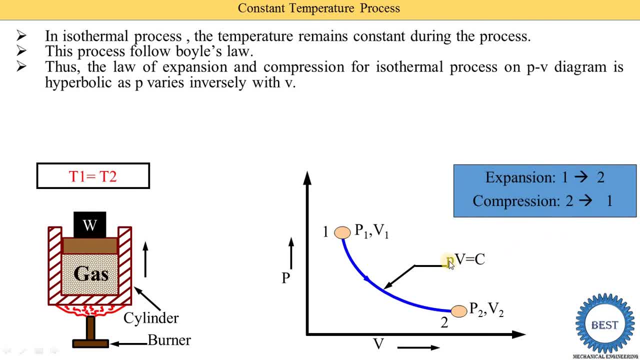 p is inversely proportional to v. okay, so v is supplied on the left side. then what we written, the pv is equal to c. okay, so this one to two is indicate. the expansion process means the. it is a heat rejection process. so in this case, here you see, in the cylinder piston arrangement, we supply. 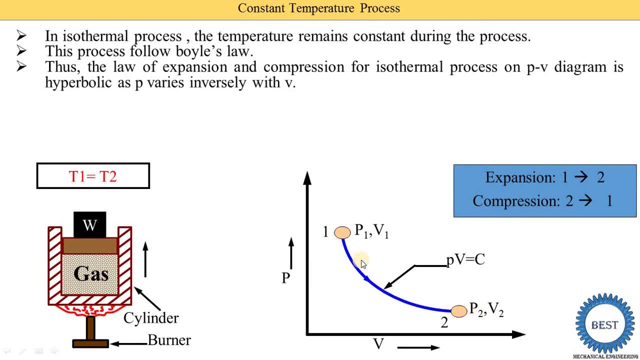 this heat energy means it is the compression process and process two to one is carried out. okay means, when we supply this heat energy, pressure is increased and volume is reduced. here you see, it is called as the compression process and second one is the one to two is the expansion process. so this process is called as the hyperbolic process. why so? 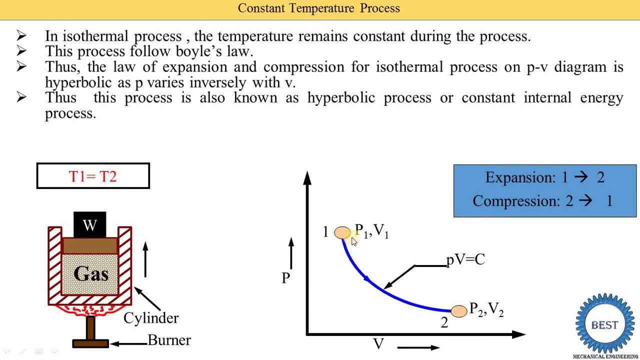 when we draw the constant temperature process on the pv diagram, we get this high curve and the curve shape is the hyperbolic. okay, that's why it is also called as the hyperbolic process and they are also called as the constant internal energy process. so why it is called as the constant internal energy process that we discuss later on when. 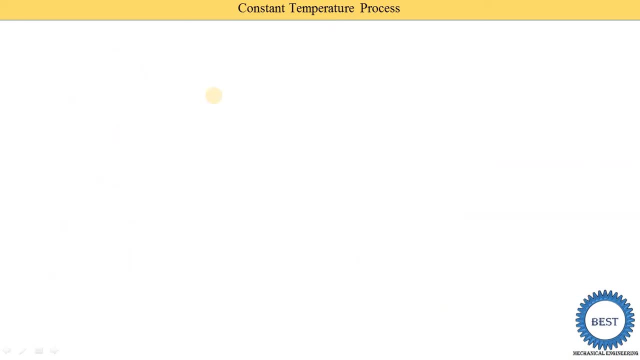 we find out these equations of the internal energy. okay, now we find out the relationship between pressure volume and temperatures. so basic equations of this pressure volume and temperature is this: that is, the p1 into v1 divided by t1 is equal to p2v2 divided by t2. so in constant. 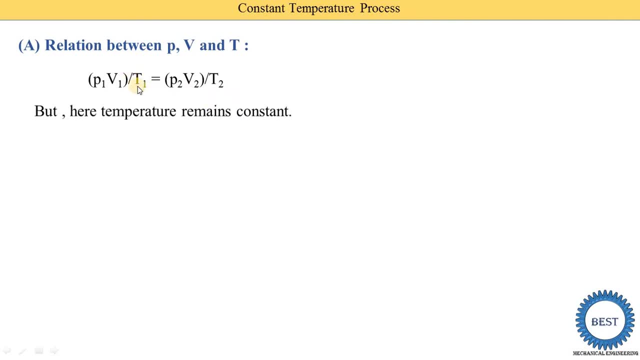 temperature process. we know that the temperature is remains constant means t1 and t2 are same. so we cancel t1 and t2. so what we get it is the p1 into v1 is equal to p2 into v2. okay, so we get this equation that means the pv is equal to c for all the stages. so it's followed a boil slow this. 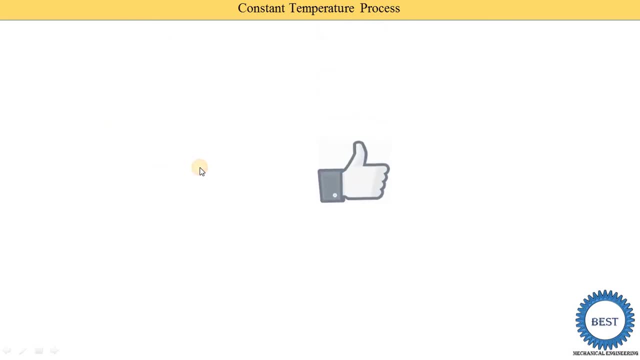 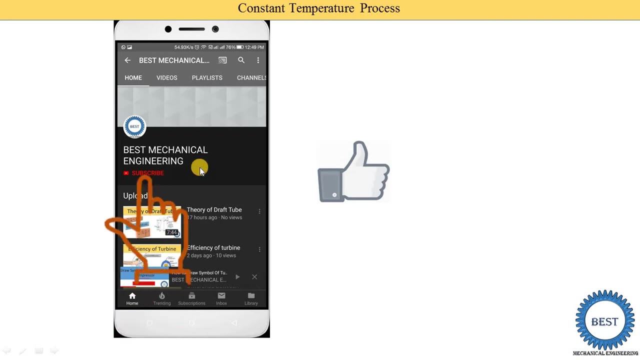 is the boil slow now. before moving ahead, i request to like the video and subscribe my channels for watching the more video related to bme subject or eme subject or engineering thermodynamics for bme or eme. various link is provided in descriptions as well as in a card for other. 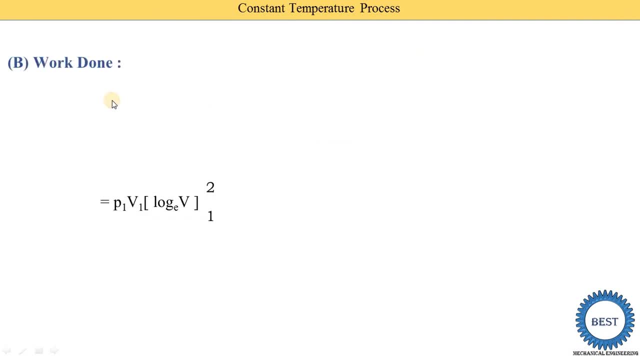 subject: i request to visit the playlist now. next, we find out this work done. okay, so work done is denoted as the w. okay, so here we return as the del w. so basic equation of the work done is the pressure into change in the volume. okay, or we also find out this work done from the pv diagram. 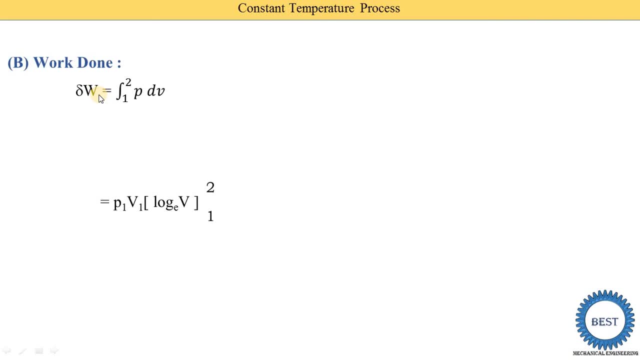 means area under the line is indicate this work done on the pv diagram. okay, okay, so here we do these integrations of the dv. okay, and we also know that the p1, v1 is equal to p2, v2. that means the pv is equal to c. so we find out some value of the pressure. 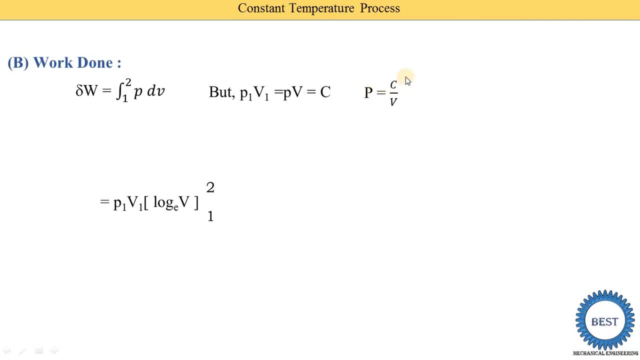 from this relationship. okay, and we get this relation. p is equal to constant divided by volume. okay, so this pressure in the equation of the work done is replaced by the c upon volume means constant upon volume. okay, so here we replace this p. then constant is constant, so we are not able to do the integration of this constant parameters, okay. 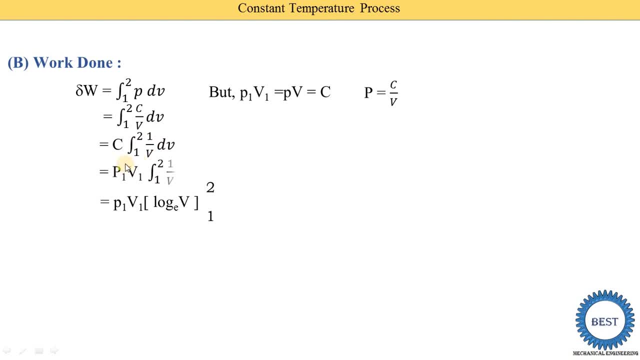 so only we do the integration of the dv upon v. then we get these equations. okay, not be getting. but here we replace the c. okay, so instance of the c, we putting this p1 v1 according to this relationship. okay, means dc constant is replaced by the p1 v1. now we do the integration of the d. 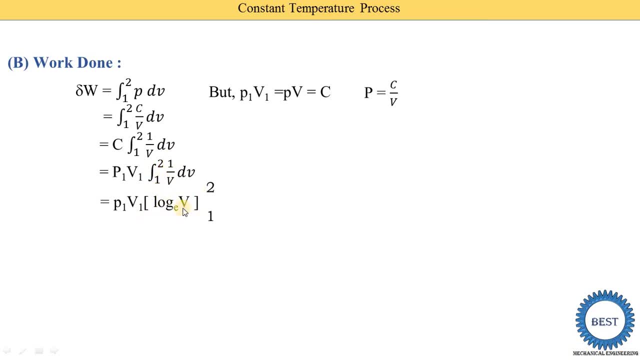 dv upon v. then we get these equations, that is a log e 1 dv upon v. okay, p1 is equal to c. recognize basic equations. that is a log e v 2 to 1. then further we simplified, we get this equation of the work done, that is a p 1 v 1 is equal to, sorry, p 1 v 1 into log e, v 2 upon v 1. okay, and in this: 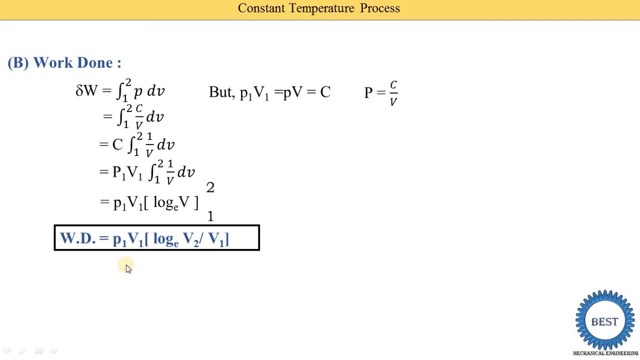 equation of the work done. we are also able to change this p 1 v 1 by the m r t 1, because we know that the p v is equal to m r t. okay, so, instance of this p 1 v 1, we are also able to. 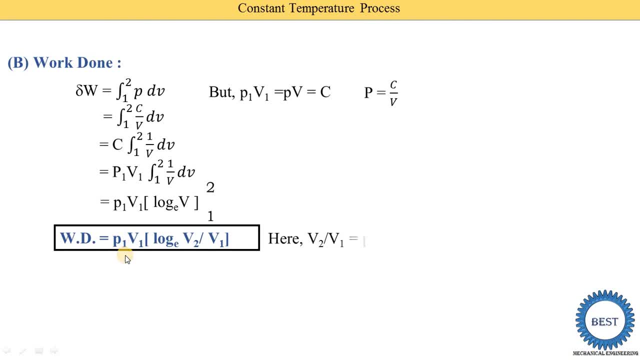 return- this is a m into r, into t 1 and, instance of this, v 2 upon v 1. we are also able to return p 1 upon p 2 because earlier in this relationship between pressure volume and temperature we find out this relation: p 1, v 1 is equal to p 2 v 2. okay, so suppose we supply this v 1 on the right. 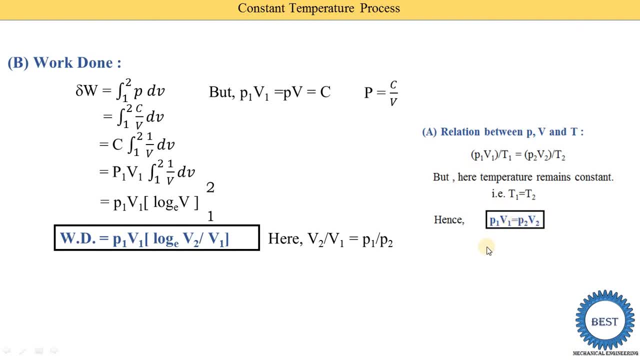 side. we get this v 2 upon v 1 and we supplied p 2 on the left side. then we get this: p 1 upon p 2 is equal to v 2 upon v 1. okay, so we are also change the equation of the work done, that is, a log e v 2 upon v 1, into log e v 2 upon p 2, and 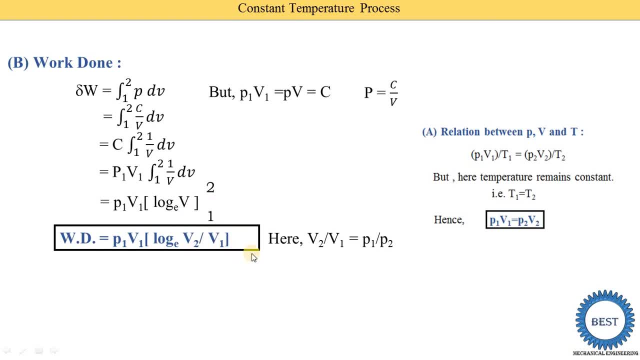 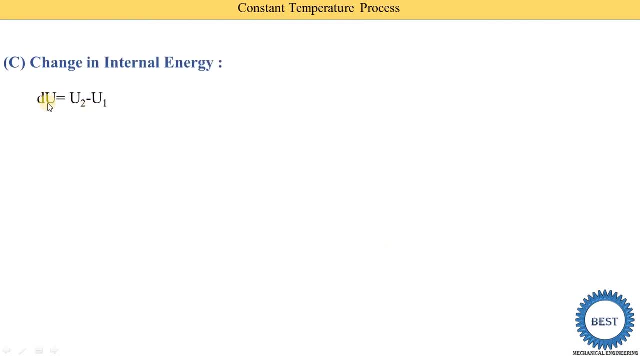 change. this value means we are able to replace this v 2 upon v 1 by the p 1 upon p 2. now next we find out change in the internal energy. so change in internal energy is denoted as the du means du is equal to u 2 minus u 1 and du is equal to m cv t 2 minus t 1. okay, so for the isothermal. 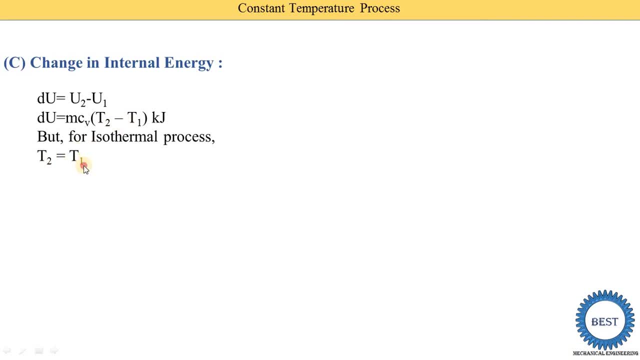 process. both the temperature are same. t 1 and t 2 are same. that means there is a change in internal energy. are zero means change in internal energy. are zero. that means this process are also called as the constant internal energy process, because that is a no change in the internal energy. okay, and no change. 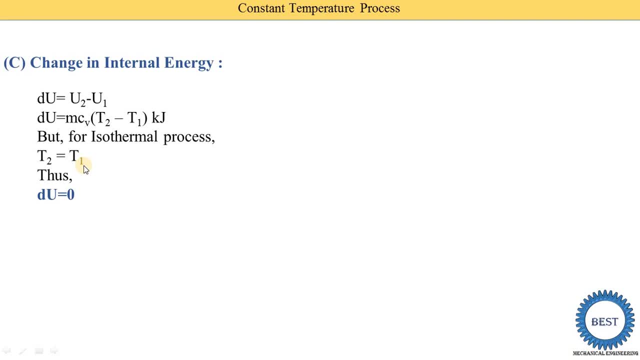 in the internal energy. that means the what amount of the heat energy we supplied. it is directly converted into the work. okay, because we know that is the equations. of the q is equal to work done plus change in the internal energy. so here change in internal energy is zero. 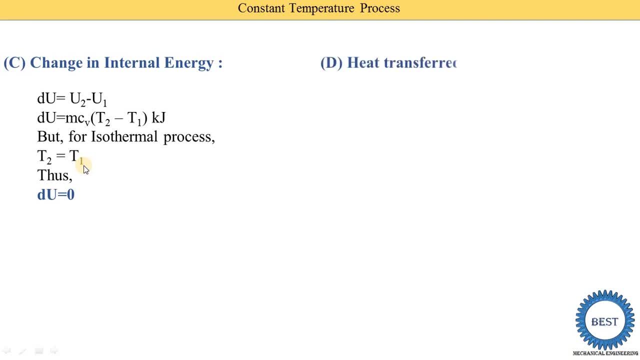 that means the work done and heat transfer are same that we discuss here. okay, in these equations of this heat transfer. so as part of first law of thermodynamics, we know that the heat supplied is equal to work done plus change in internal energy. so here what we find out: internal energy is zero. 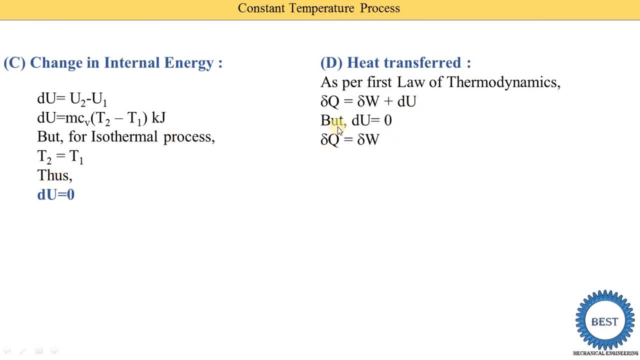 okay, so this du is equal to zero. then what we get heat supplied is equal to work done. okay, and we also know the equations of the work done. okay, so we are directly written these equation: p1, v1, log e, v2 upon v1 instance of this p1, v1. we are also able to return mrt1. okay, so we. 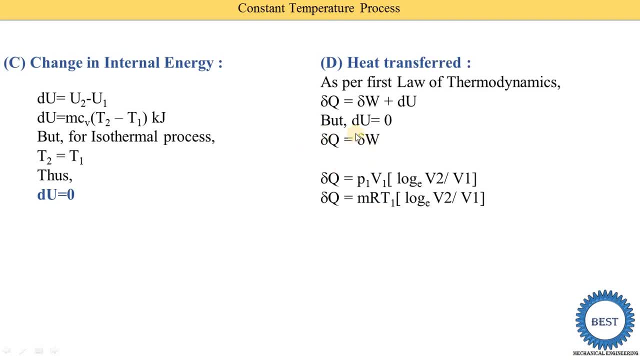 getting these equations of the heat transfer. okay means in a constant temperature process the internal energy is zero and heat supplied is 100 percent converted into this work energy. okay. if we consider the other losses are zero. change in enthalpy. so equations of the change in enthalpy. 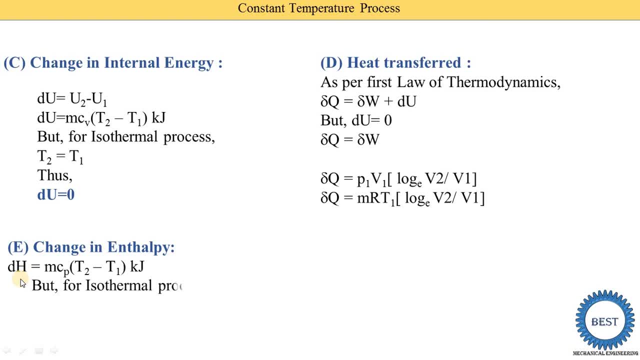 is the mcp t2 minus t1. so we know that it is isothermal process. temperature are same, t2 is equal to t1, so enthalpy change in the enthalpy is also zero. okay, so during the constant temperature process, internal energy are zero, change in enthalpy are zero and the heat interaction is. 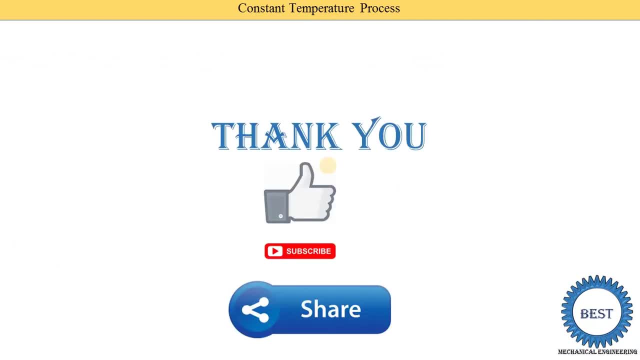 equal to work interactions. so thank you for watching this video. if you learn something, then like the video, subscribe my channel and don't forget to share with your friends. 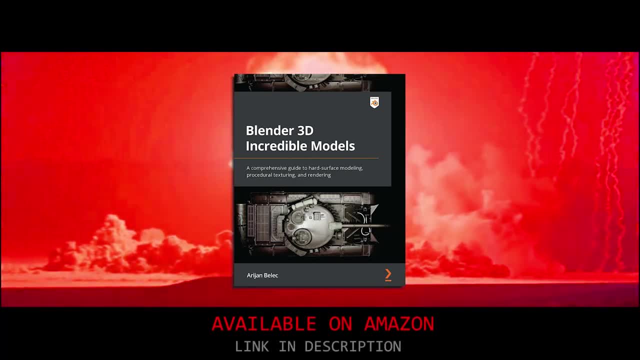 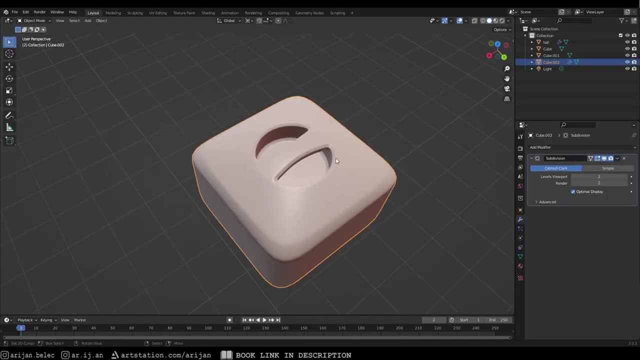 All right, I have a little topology exercise for you guys, which I pulled out out of my little topology guide that I'm writing and that's going to be available to you guys soon, by the way. But the exercise is this little handle right here and I want to see how many of you guys can. 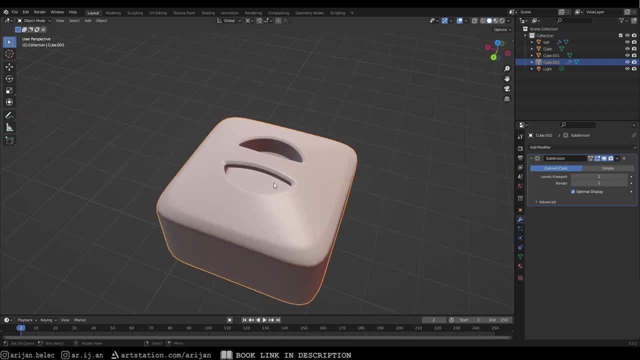 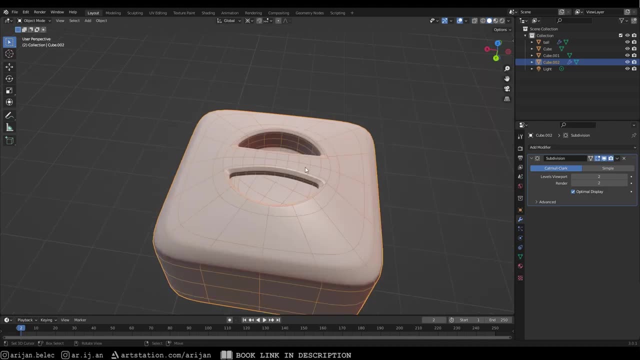 actually make an object like this with a hole and a handle or a bridge going over it, with correct topology. okay, Let me show you a little bit more closely what I mean by this. I'm going to turn my wireframe over here. as you can see, All the topology is flowing perfectly well. We have a. 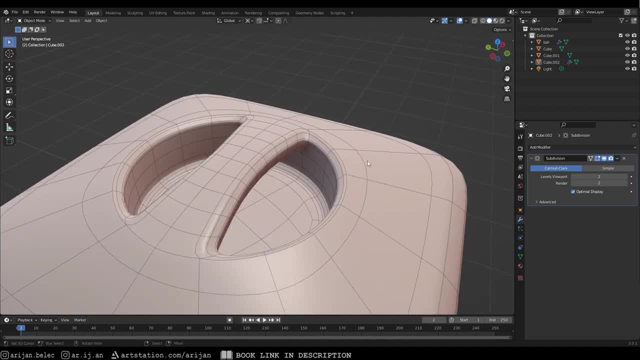 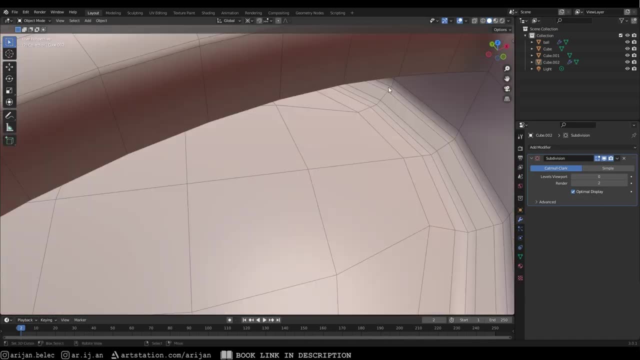 little bridge going over here. There's no triangles. I have a subdivision surface modifier over here, but if I disable that, you'll see there's no triangles, It's only quads everywhere and everything is flowing perfectly well. We have everything connected perfectly And I'm 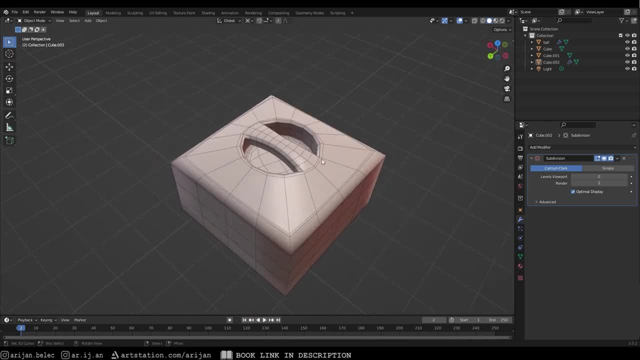 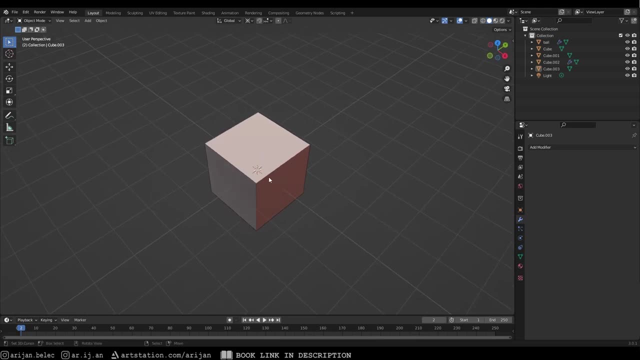 wondering how many of you guys can do this, And if it's not that many, then stick around, because that's what we're about to do here today. Now, in the previous topology tutorial, we were talking about how to make a hole in this cube correctly. all right, And there? 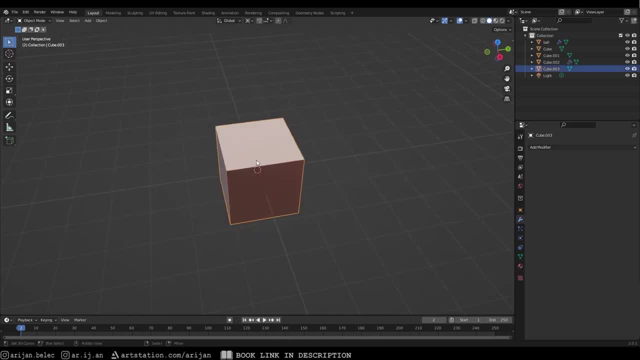 we were using some loop cuts To make a hole here without using a Boolean modifier. okay, So we're going to have to start with something similar to that here today. okay, So the first thing that we have to do with this cube is we have to select it in edit mode and we have to subdivide it a couple of times. 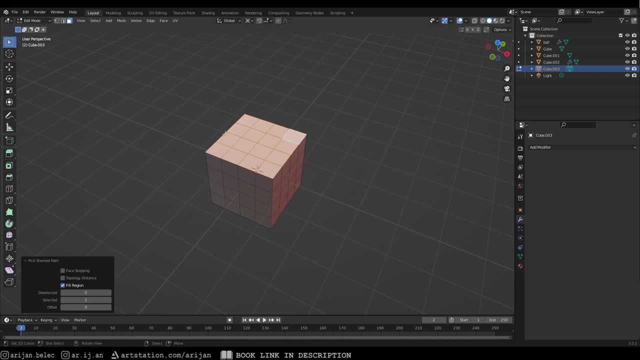 Now keep in mind, the more that we've subdivided, the more squares we have up here to form a circle, which means our circle is going to have a little bit more polygons. It's going to look a little bit smoother, right, So you can go further than this. You can subdivide it once more if you want.